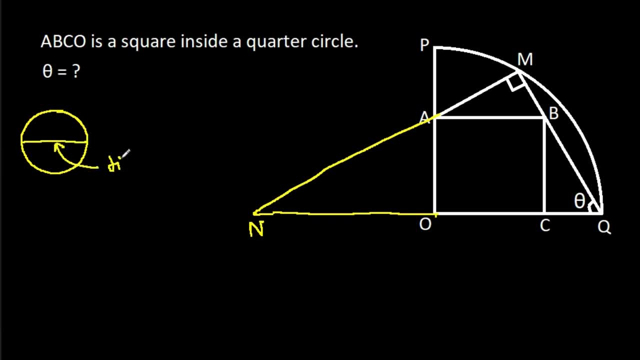 diameter makes an angle of 90 degree on the circle, And here we have angle. QMN is equal to 90 degree. So QN it will be 90 degree, QN it will be diameter, QN. it will be diameter. 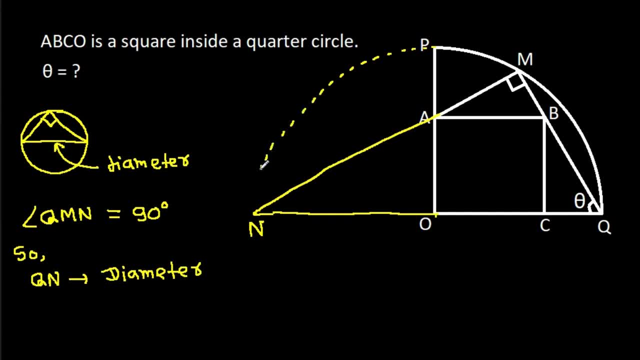 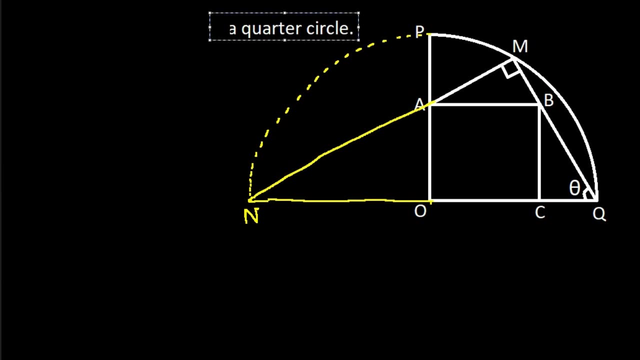 And now interangle QMN. it is QMN. This angle is 90 degree. This angle is theta. So this angle, it will be 180 degree minus 90 degree minus theta. That will be 90 degree minus theta. It is 90 degree minus theta. 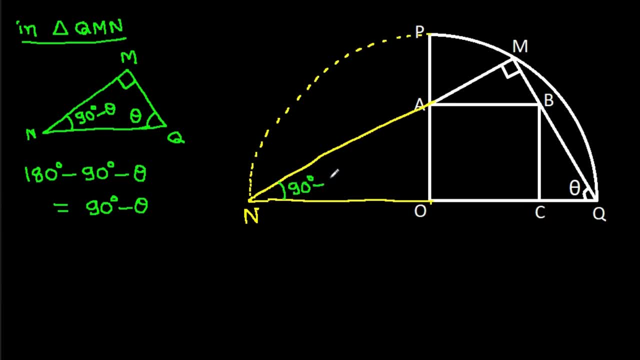 This angle it is 90 degree minus theta, And we know that ABCO it is a square. That means these angles they will be 90 degree minus 90 degree minus theta. So this angle it will be also 90 degree, And this angle it will be also 90 degree. 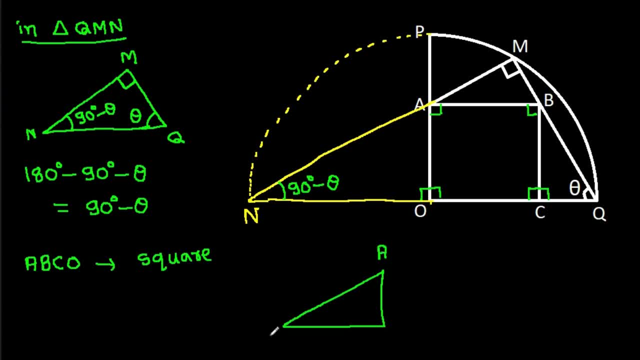 And interangle ANO. this angle is 90 degree. This angle is 90 degree minus theta. So this angle, it will be 180 degree minus 90 degree, minus 90 degree minus theta. That will be theta, It will be theta, This angle, it will be theta. 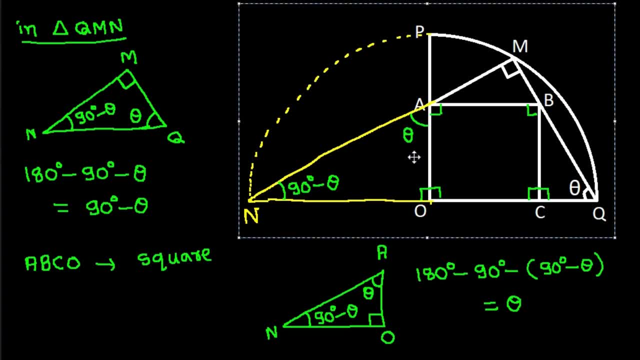 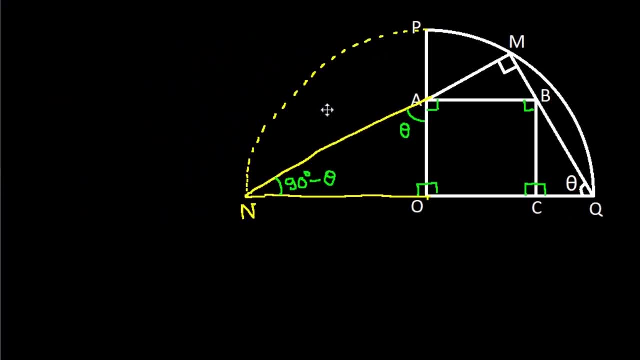 And now that angle will also be 90 degree, Because there will be angle not always, So think that angle. it will be just 90 degree. That is the general answer. what in someone will get is equal to angle AON, that is, 90 degree, and angle CQB it is equal to angle OAN, that is theta. 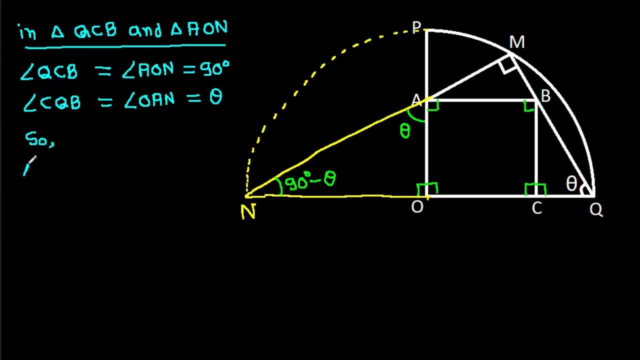 So the angle QCB it will be similar to the angle AON. Hence QC over AO it will be equal to CB over ON. So QC is the angle of A and we know that QN it is diameter. So OAN it will be equal to OQ. that will be radius. 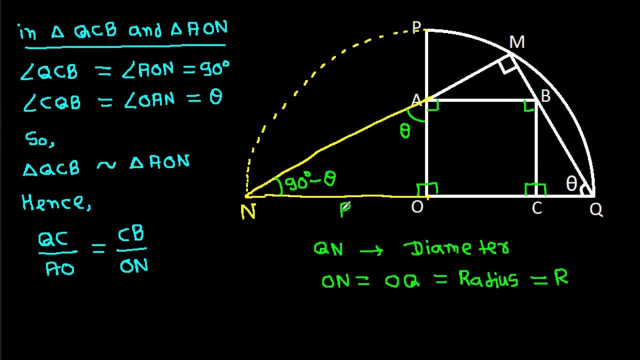 Suppose R, OAN is R and OQ is r and we know that abco it is a square, that means ao. it will be equal to ab, it will be equal to bc, it will be equal to co. suppose a, ao is a, bc is a and co is a, and we know that oq is r, so cq it will be r minus a. 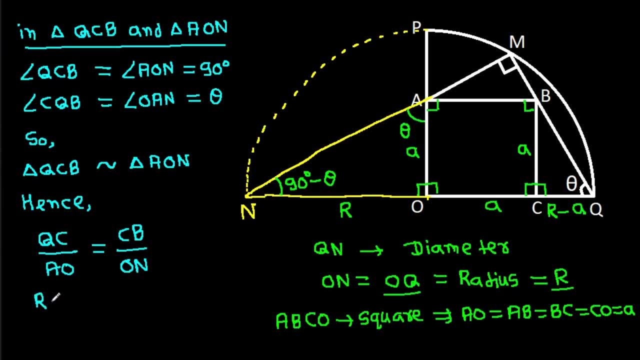 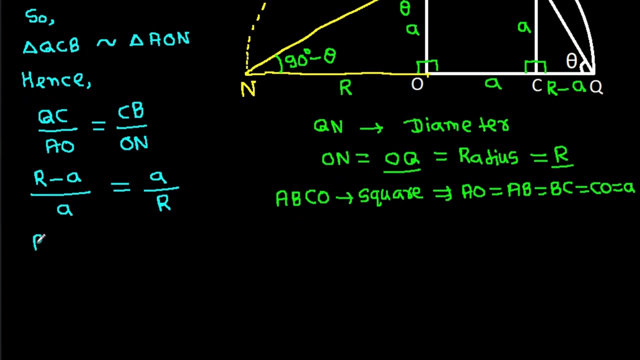 so qc. it is r minus a over ao is A. it is equal to CB. it is A over ON is R and it is R over A minus A over A is equal to A over R, and it is R over A minus A over A, it will be 1, that is equal to A over R. 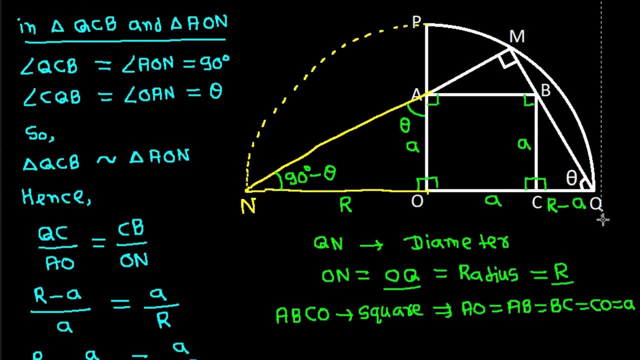 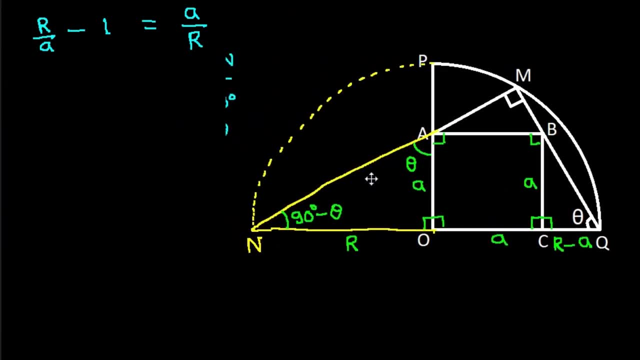 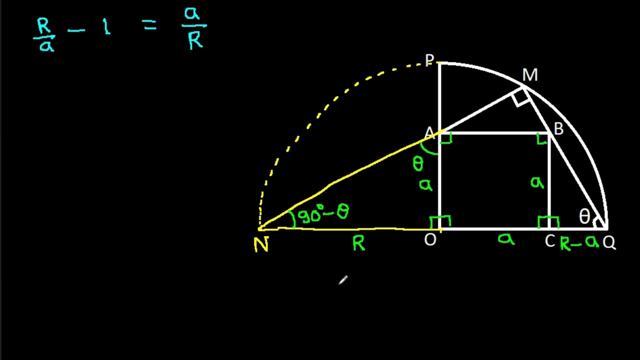 and Now in triangle: AON. this angle is 90 Degree. this angle is Theta, ON is R and AO is A, so tan Theta, it will be ON over AO and ON is. 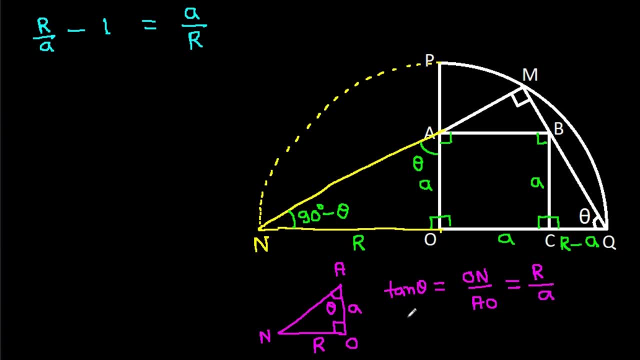 R over AO, AO is A, So R over A it is tan theta minus 1, it is equal to, and A over R it will be 1 over tan theta, And if we cross multiply, then tan theta times tan theta. 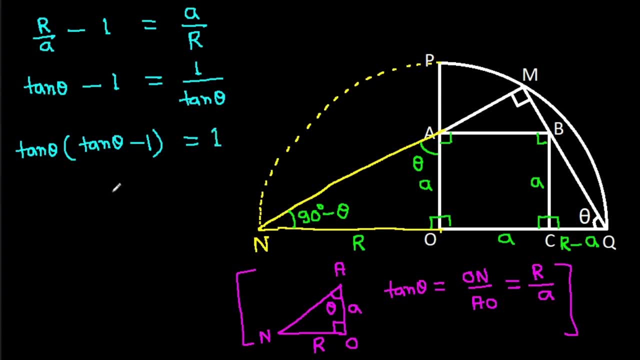 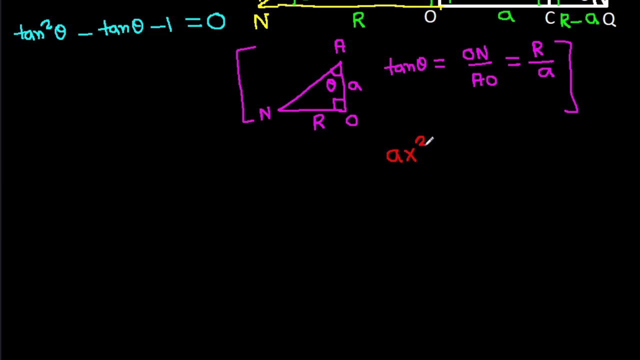 minus 1, it will be equal to 1.. And it is tan square theta minus tan theta is equal to 1.. And tan square theta minus tan theta minus 1, it will be equal to 0.. And for equation AX square minus BX, minus C is equal to 0.. X is equal to minus B minus minus root under. 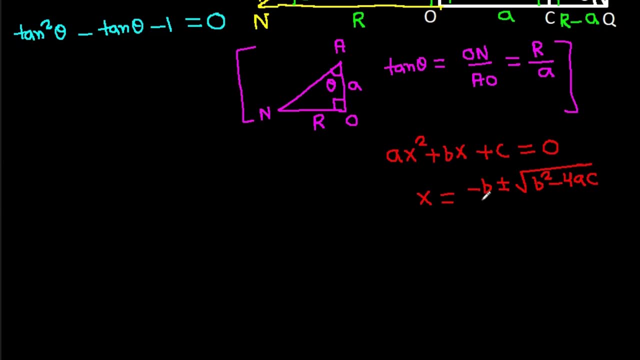 B square minus 4AC over 2A, And here A is 1,, B is minus 1, and C is minus 1.. So we will get tan theta minus 1.. So tan theta, it will be minus, and B is minus 1, minus. 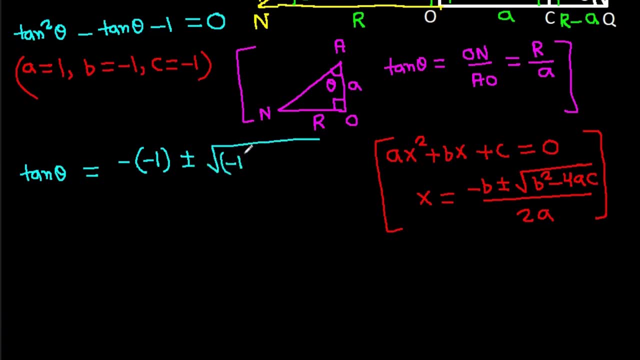 minus root under B is minus 1,. A square minus 4 times A is 1, and C is minus 1 over 2 times A is 1.. And tan theta: it is 1 plus. minus root under 1 plus 4 over 2.. And tan theta, it is 1 plus. 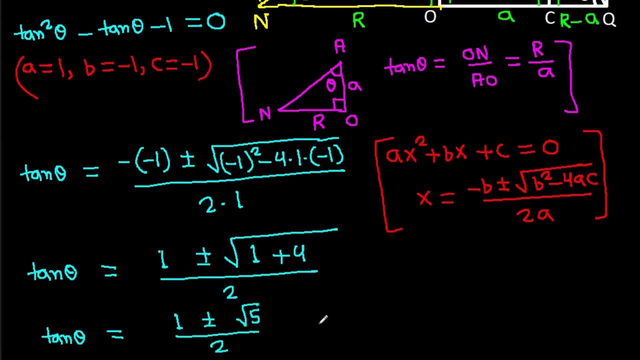 minus root, 5 over 2.. And tan theta, it is 1 plus minus root, 5 over 2.の tan pose Statia, It is 1 plus minus root, 5 over 2.. And tan theta, it is 1 plus minus root, 5 over 2.. And tan. theta, it is 1 plus minus root, 5 over 2.. And tan theta it is 1 plus minus root, 5 over 2.. And R over A it is Vamos. So this is: 1- LA, memorize, Geo, and then R over IS, and then zodiac. R over A. A is 1-ALP, So this is B and G, where this experienced S shouted 1 uh S, Uh Long on 지 dan обязih. Now and see what do Dan says. C' how does a Ta z 그래도 Tasiah? 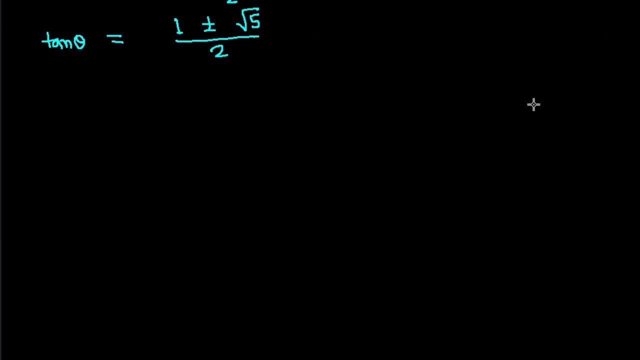 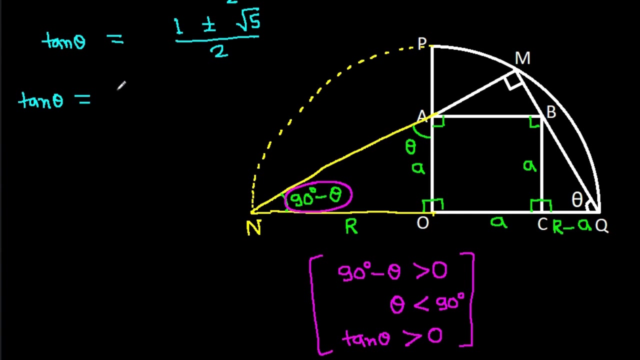 90 degree minus theta, it should be positive. 90 degree minus theta, it should be positive. so theta it should be less than 90 degree. so tan theta, it should be positive. and here we get: tan theta is 1 plus root, 5 over 2, and tan theta it is 1 minus root, 5 over 2, so tan.